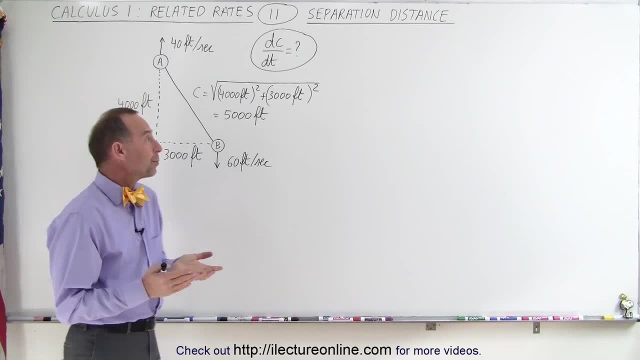 Welcome to my lecture online Here. our next problem: we have two cars- let's label them A and B- who are driving away from each other, but not directly away from each other. They're offset by 3,000 feet. They're currently 4,000 feet in the north-south direction away from each other. Car A: 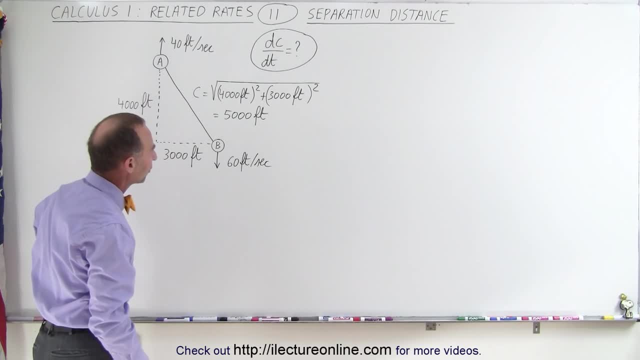 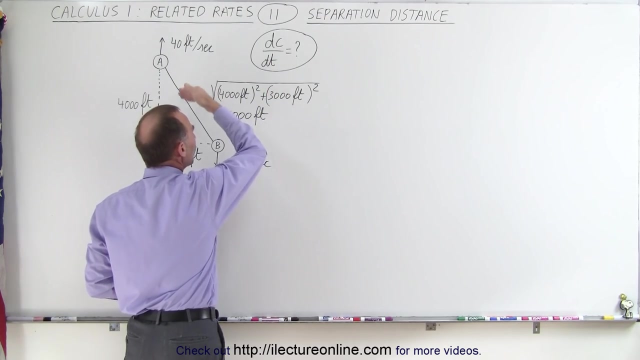 is driving 40 feet per second in the northerly direction, Car B is driving 60 feet per second in the southerly direction and at the moment that they're 5,000 feet apart- because we can calculate the 5,000 feet from using Pythagorean theorem- we want to figure out how fast the distance between 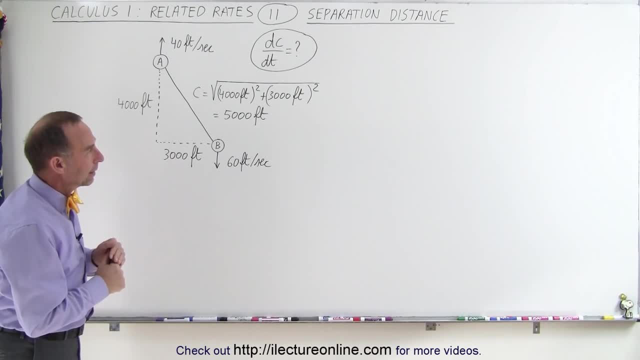 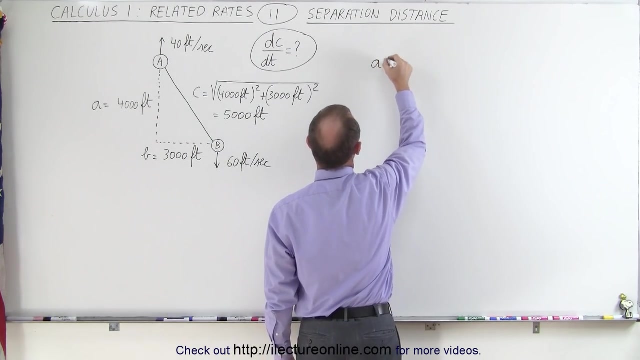 them is changing at that very moment in time. All right, the way to do that is we need to find a relationship between the sides and the hypotenuse. Let's call this side A and let's call this side B, and so what we could say is we could say that A squared plus B squared, equal C squared, Of course. 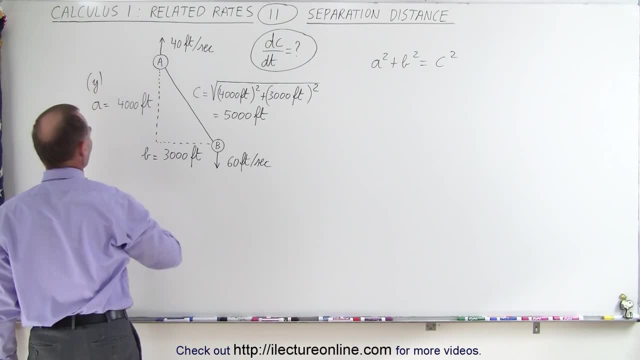 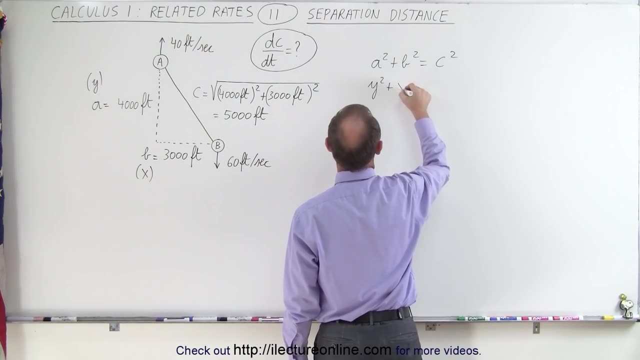 we could use the variable Y for the vertical direction and we can use the variable X. so in this case we can say: A would be Y squared plus X squared is equal to C squared. So we could also write it like that. Okay, what we want. 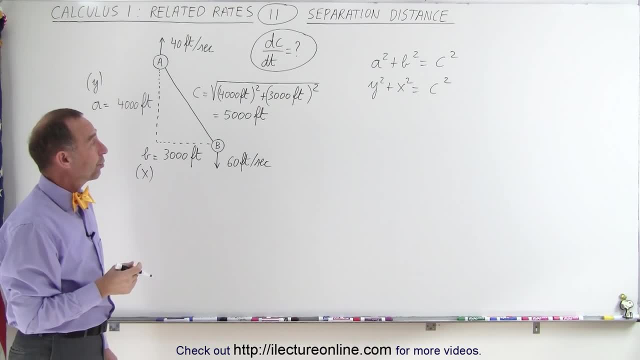 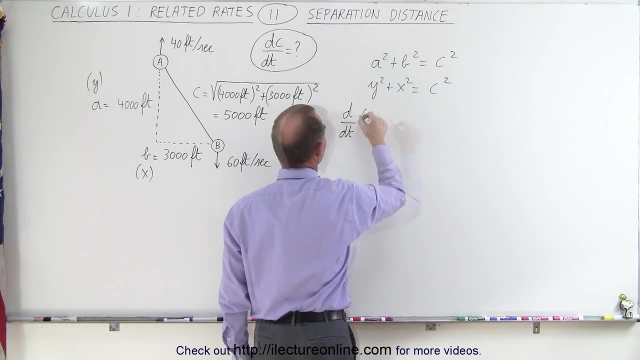 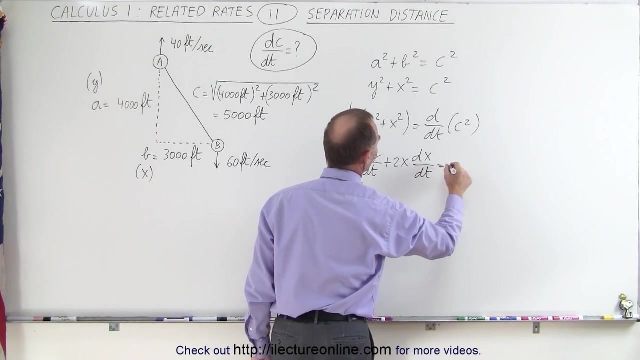 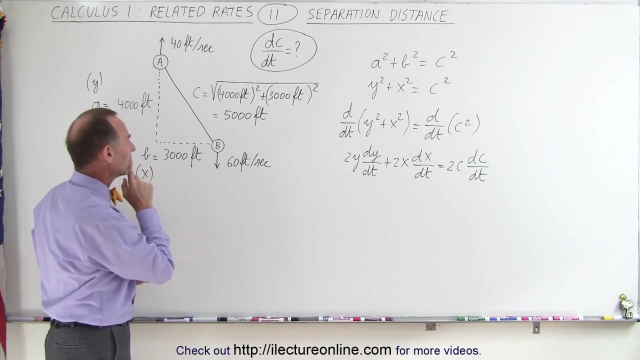 to do now is take the derivative of both sides, which with respect to time, so we can find dc dt in there. So let's do that. the d dt of the left side is equal to the d dt of the right side. So this gives us 2y dy dt plus 2x dx dt is equal to 2c times dc dt. So right away we can see here that there's 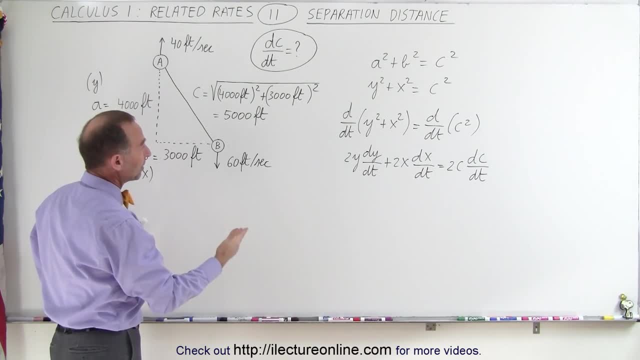 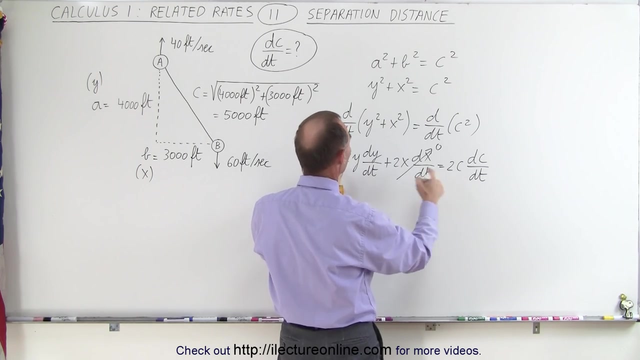 no movement in the horizontal direction or the x direction. That means that dx dt must be equal zero. There's only movement in the y direction, so we only have a dy dt. So that means that this term disappears. This is equal to zero, and we can also see that both sides of the equation can be.